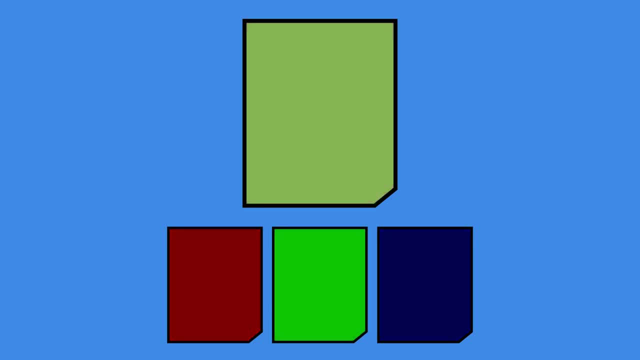 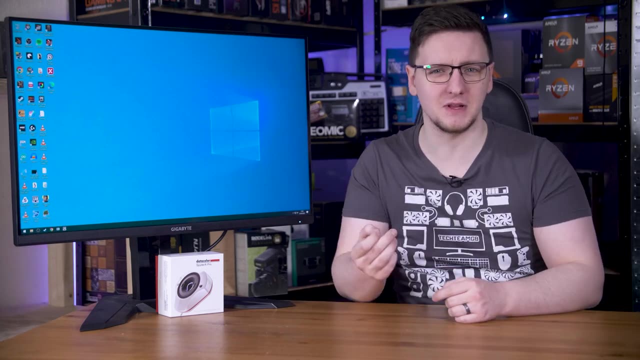 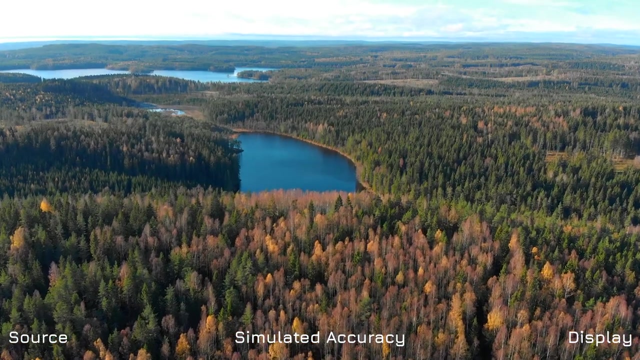 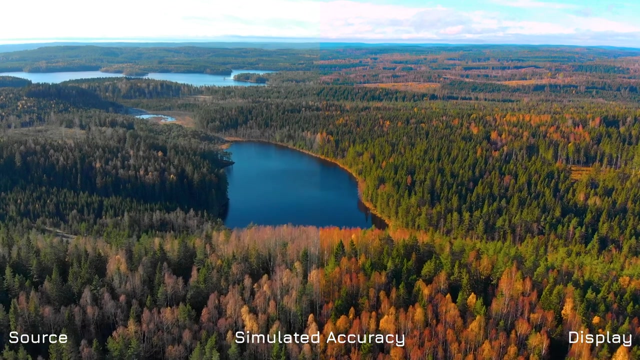 of colours without needing a way to produce more than three of them. Colour accuracy is pretty simple: It's how close your screen gets to displaying any given colour correctly. A very colour accurate display will display colours imperceptibly close to the actual colour you expect, whereas an inaccurate display 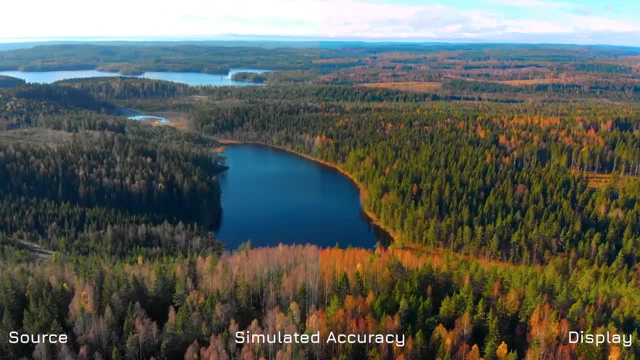 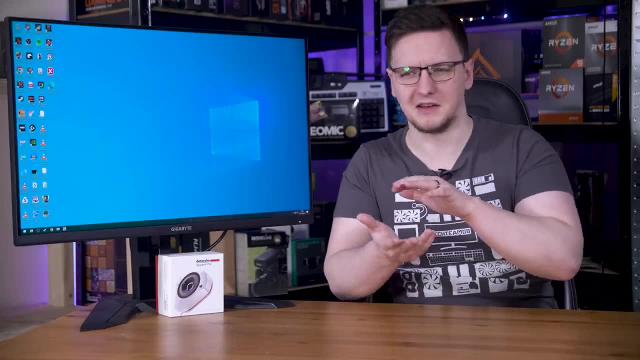 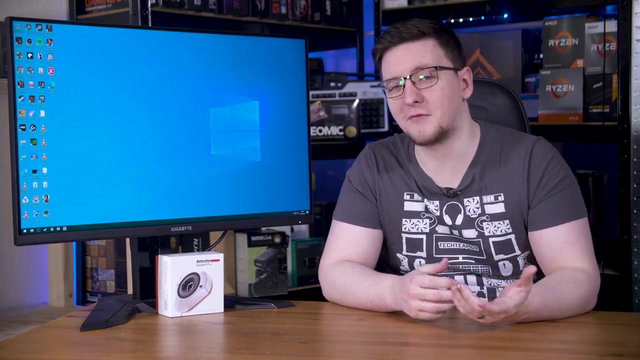 will show you colours that are wildly different from what you should be seeing. The way this is measured is with a value called Delta E. with the lower the Delta E, the more accurate the colour is. If you picture the whole visible light spectrum on a graph, you'd get something like this: 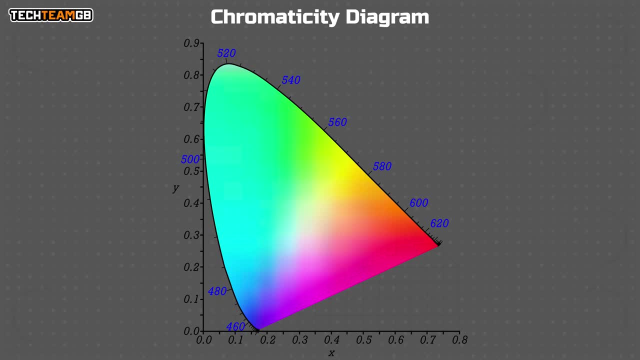 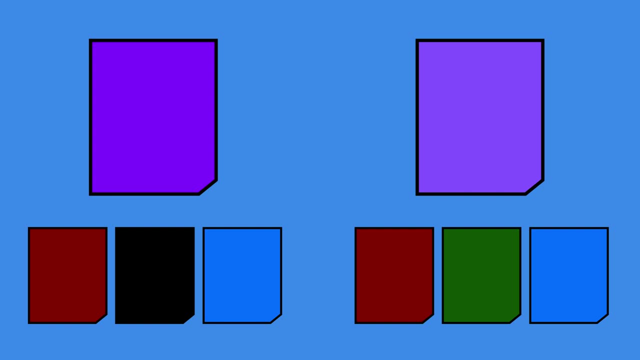 a chromaticity graph If your monitor tries to display, say, this purple colour, but it ends up leaking a bit of green light, so you end up with more like this shade instead. well, that's not a very accurate rendition and therefore would have a higher Delta E value. 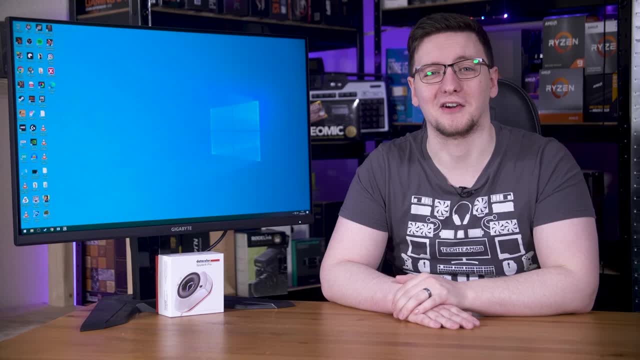 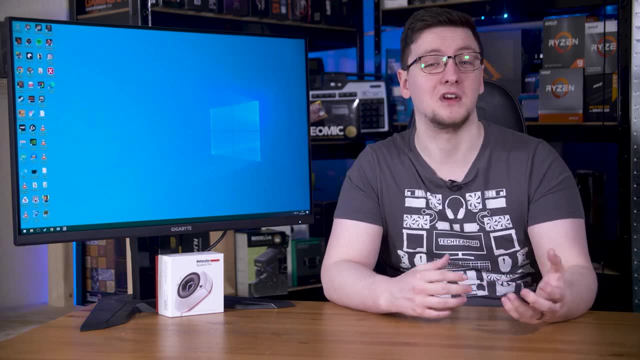 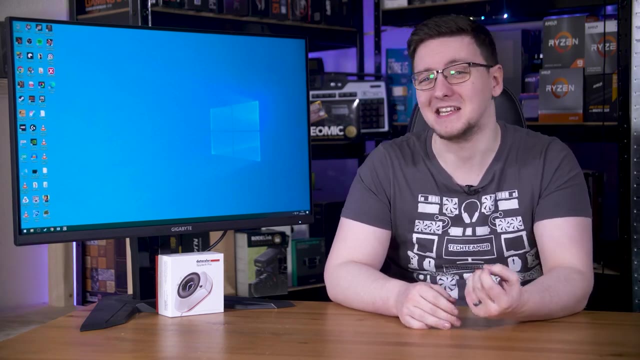 Now, Delta E is a remarkably complicated calculation and there's actually been multiple versions of the figure. CIE, the International Commission on Illumination, an over-century-old company, has been working on this figure for over a decade. The old organisation first offered Delta E in 1976 as just the Euclidean distance formula. 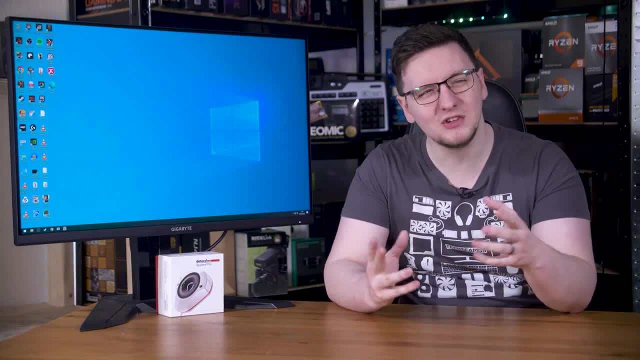 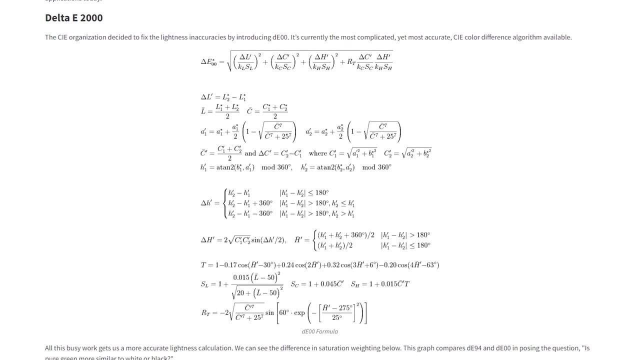 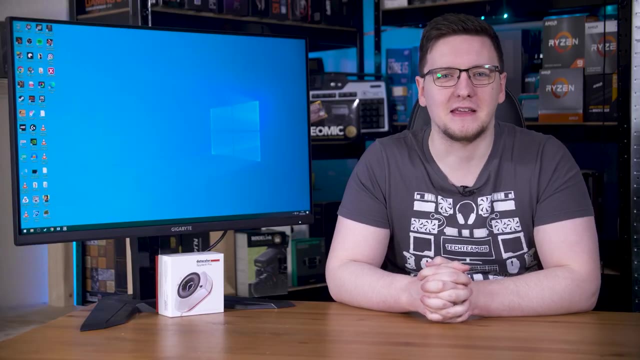 That had some problems, especially with saturation, and, in short, it was revised twice, settling with this monstrosity Delta E 2000,. which is an absolute mess. but that's how you actually calculate Delta E these days. so forgive me if I don't give you any actual numbers for my hypothetical. 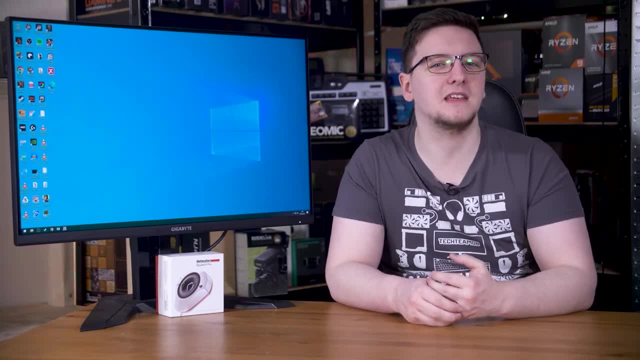 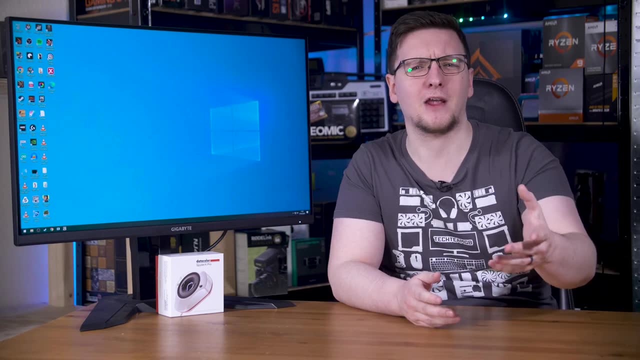 examples. Still, the rule of thumb is that a Delta E of less than 2 is what you're after for an accurate-to-the-eye display. Ideally, a panel would just perfectly reproduce all colours, but of course, the real world is far from the ideal world. 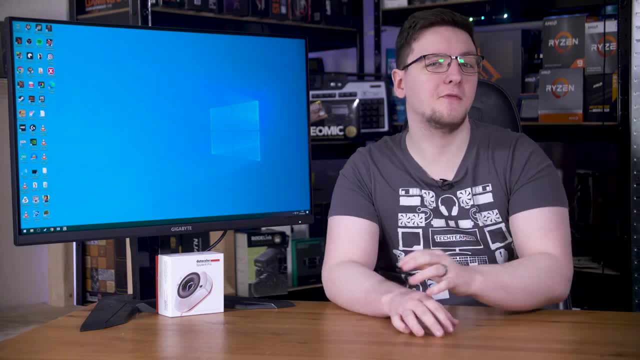 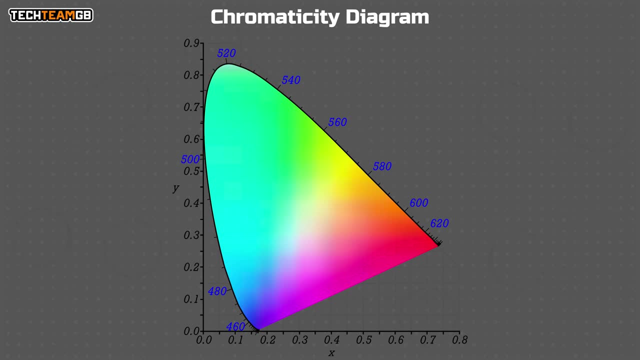 So what about this whole colour space talk? Well, if we take a look at our visible light chart here, not all of this can be displayed by monitors. There is an almost infinite number of monitors. There is an almost infinite number of monitors. 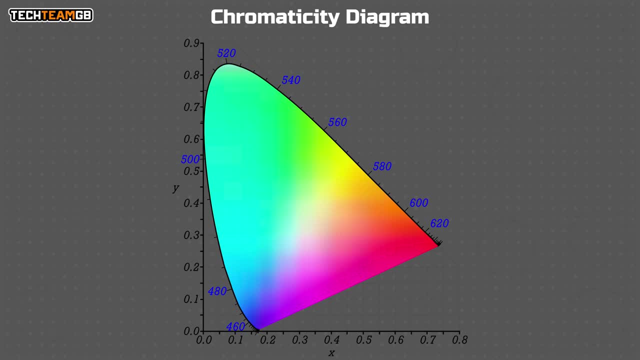 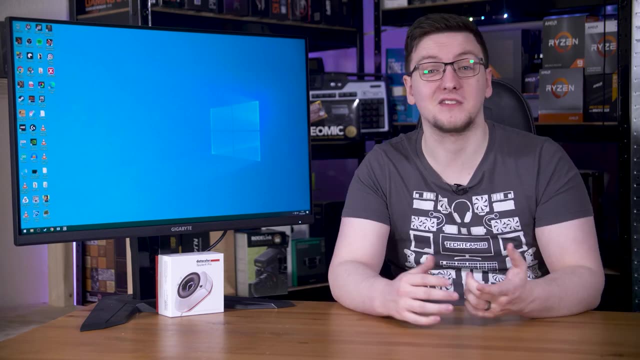 There is an almost infinite number of shades here that you could pick from. so the IEC, the International Electrotechnical Commission- yes, there's another one- standardised the sRGB colour space that Microsoft and HP had been using since 1996 as the beautifully named 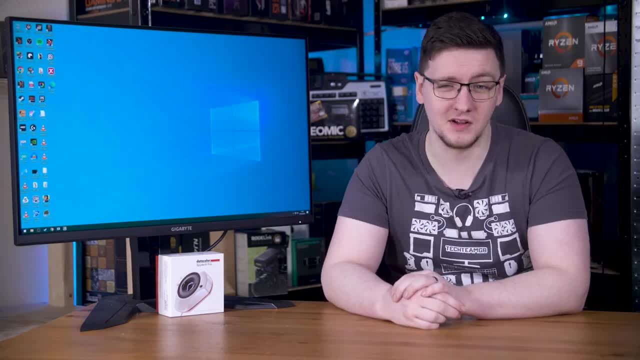 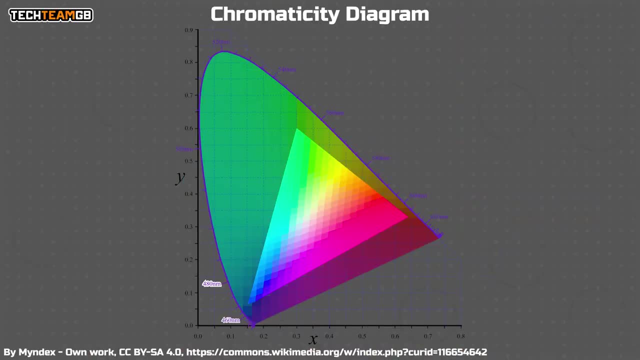 IEC 61966-2-1 standard. Yeah, I'll be sticking with sRGB. it's a bit more catchy for me Now. sRGB is one of the smallest colour spaces, but it is the standard colour that we can is the standard for web content. It's obviously made up of red, green and blue values, although 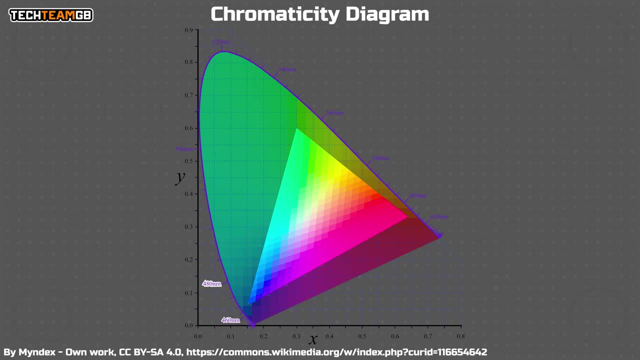 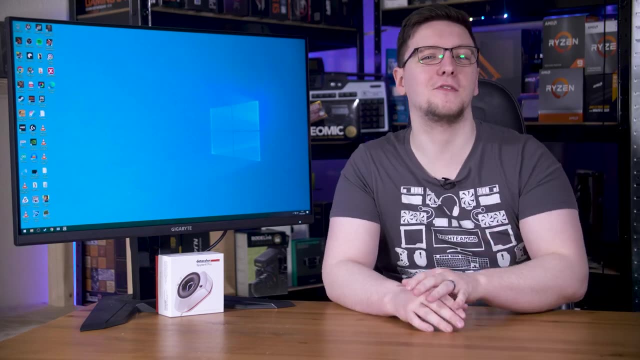 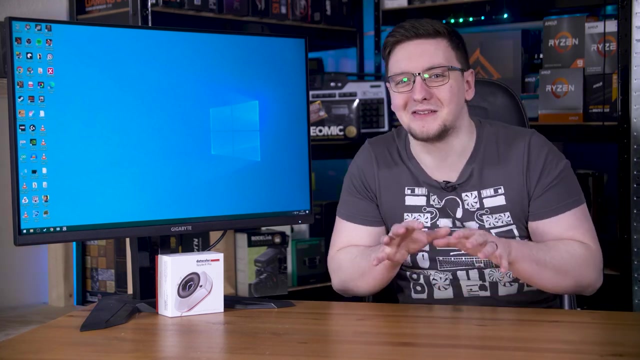 generally those values are represented as an 8-bit binary byte per colour channel. That's called 8 bits per channel and means that you have 256 different values per colour for a total of around 16.77 million combinations. As an aside, you might have noticed the setting for limited dynamic. 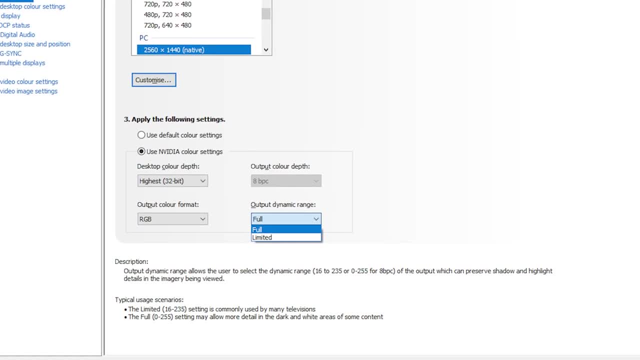 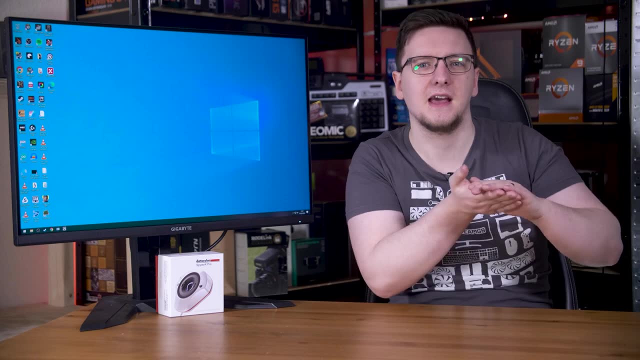 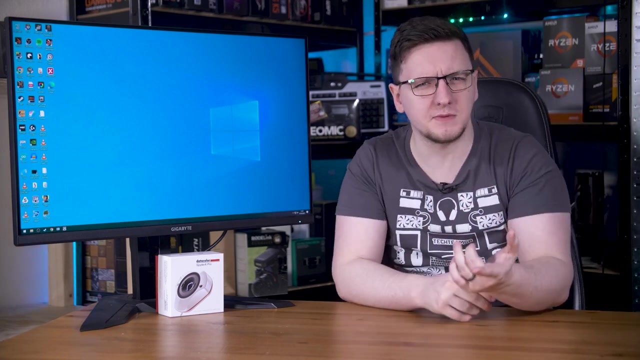 range. That is when your graphics card will artificially clip the values to RGB16 on the low end instead of down to RGB0 or full black and RGB235 on the high end. so the lighter shades instead of 255.. For most monitors you want the full dynamic range setting, but some especially. 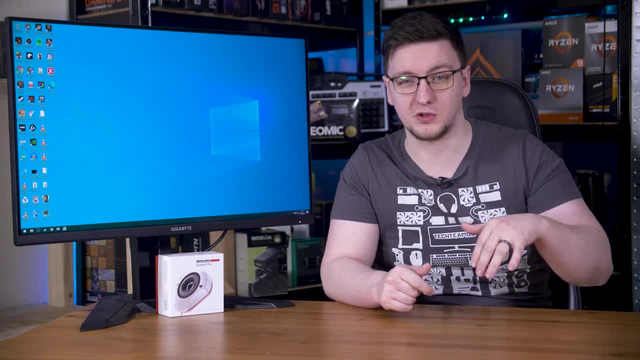 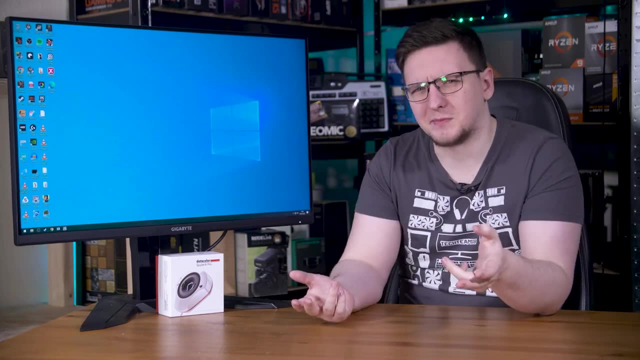 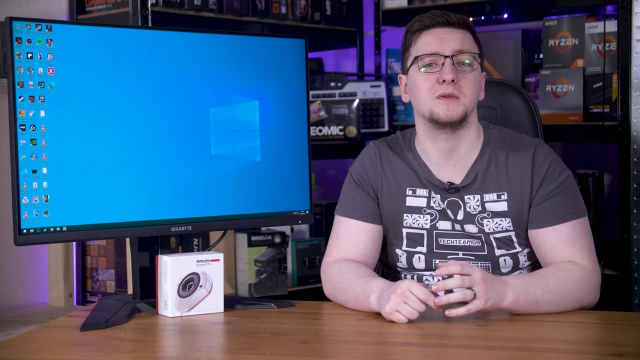 older TVs won't display RGB0 or 255 or that sort of range, right, so you need to set it to the limited range setting instead. So what about the other colour spaces? Well, the Adobe RGB and DCI-P3 spaces are much wider, with Adobe RGB being based on all of the colours that a CMYK printer can. 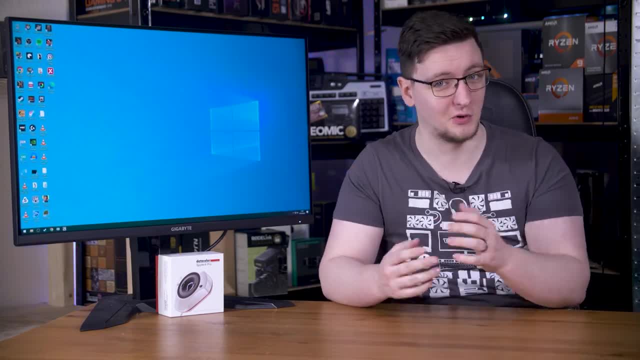 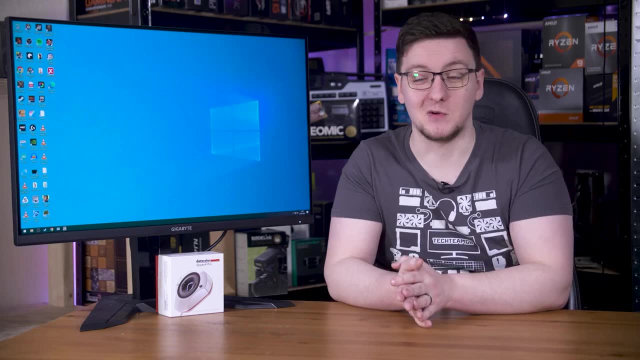 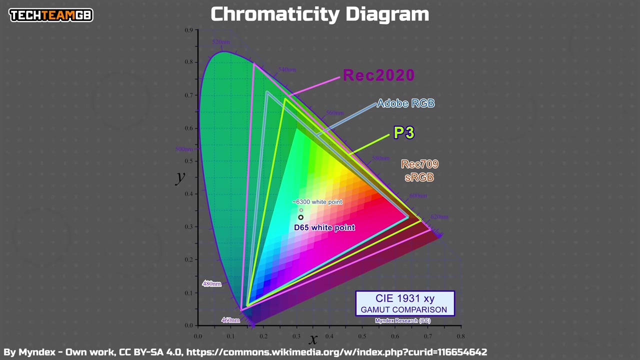 output, since, as you'd expect, the sort of people who use Adobe software like Photoshop normally want to print their work, and it would be great if they could see what colour their work is going to be before they actually print it. DCI-P3 is from DCI, the digital cinema initiative, which is what you hear more about in the video. 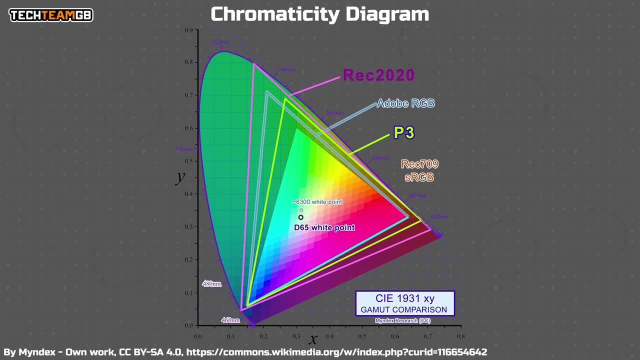 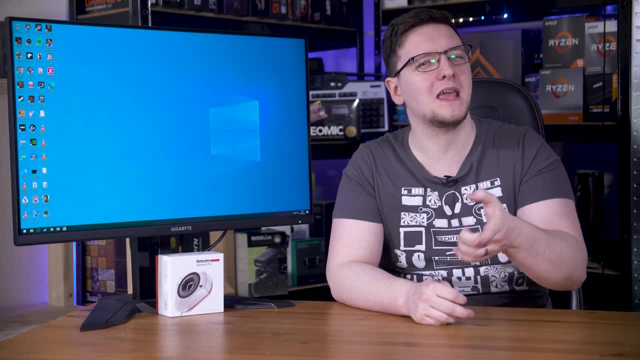 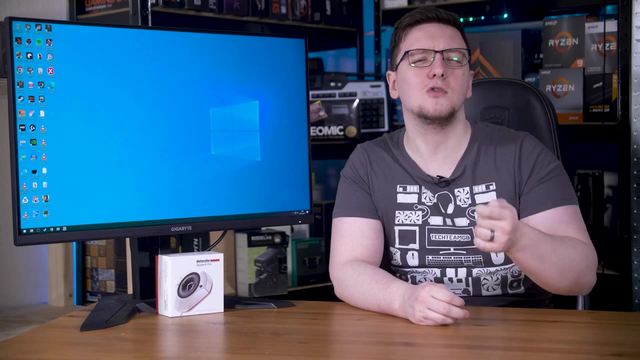 editing space and stretches into deep reds and lighter greens, compared to Adobe RGB's focus on exclusively more green. Often. to be able to display more than the 16.77 million colours SRGB usually offers, you need to use more bits per channel. Most colour-focused 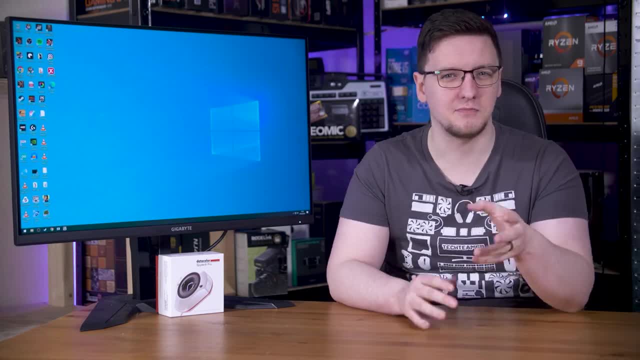 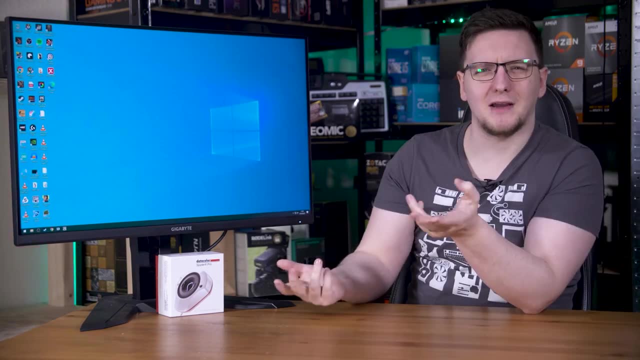 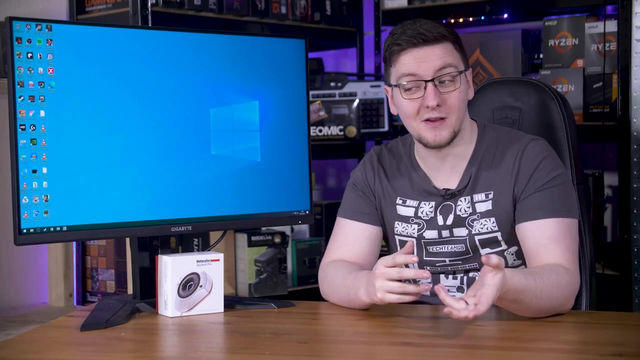 displays always offer estabanaaam 10 bits per channel, which means they have over a billion color combinations available to them. Quite an upgrade. So then, how do you test for both the accuracy and color gamut coverage? Well, that starts with a way of accurately recording what colors your display is outputting. 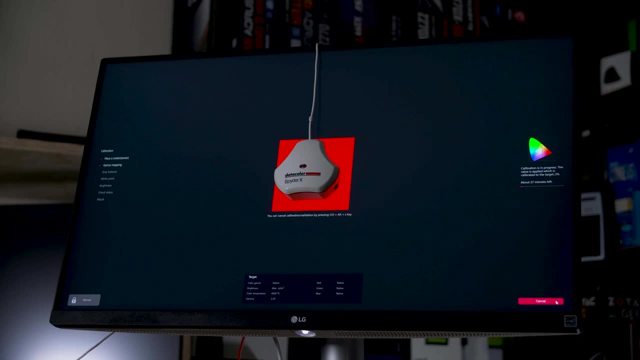 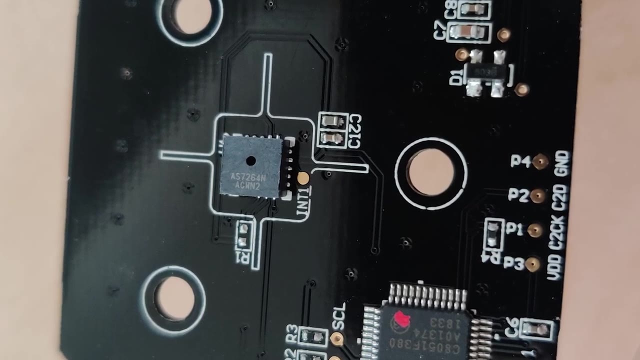 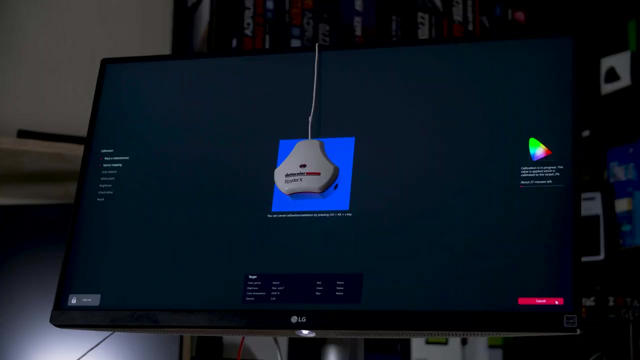 A device like this. the Datacolor Spyder X- which is not sponsored, by the way, this is just what I have available- has a 6-axis color sensor inside that acts a bit like a camera to capture how much red, green and blue light is being emitted. Their test software then has the 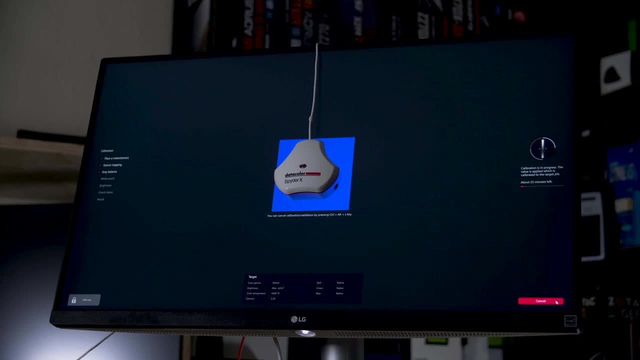 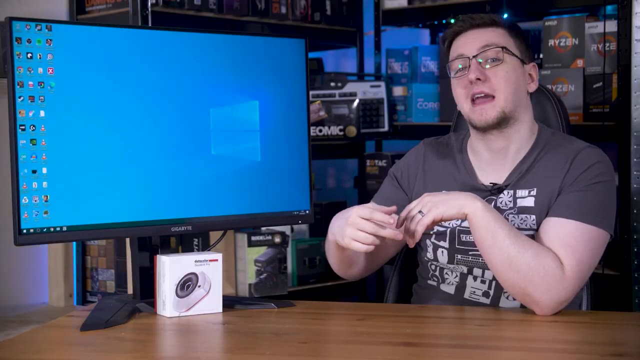 display show various colors to measure both the gamut coverage and, in a separate test, the accuracy too. You might have also heard about color calibration. It's a very useful tool, but it is important to remember that color calibration is a very important part of color calibration. It's a 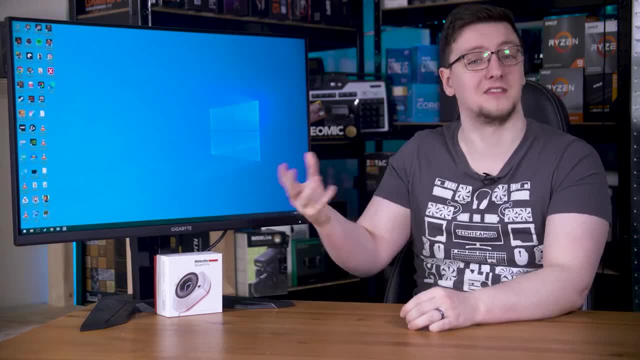 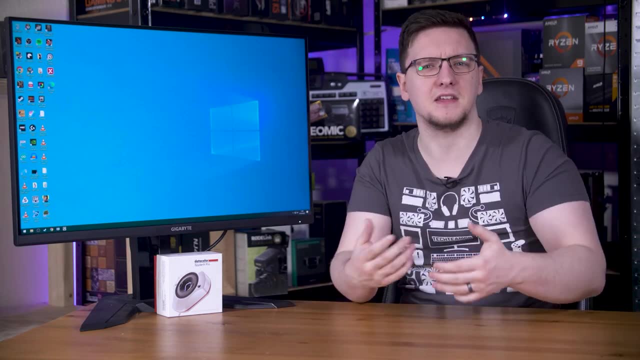 very important step to make sure you're measuring the perfect range of color, as you can see. It's also important to know that, unless the profile is stored on the monitor, the scaler itself, like some LG models, it is your graphics card, your PC, that is applying the changes to what you see. 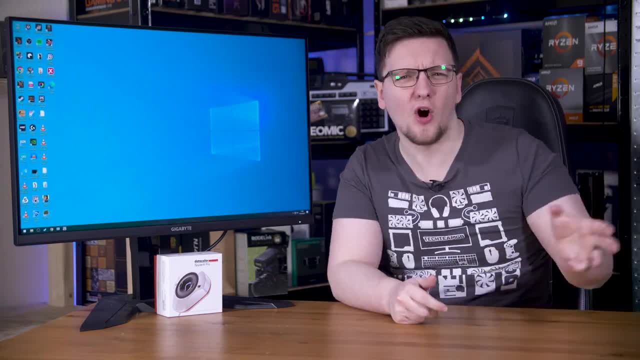 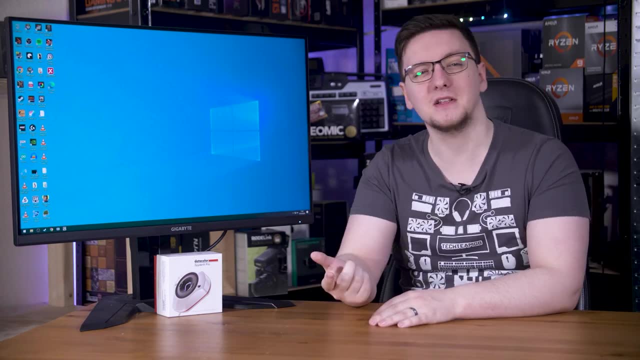 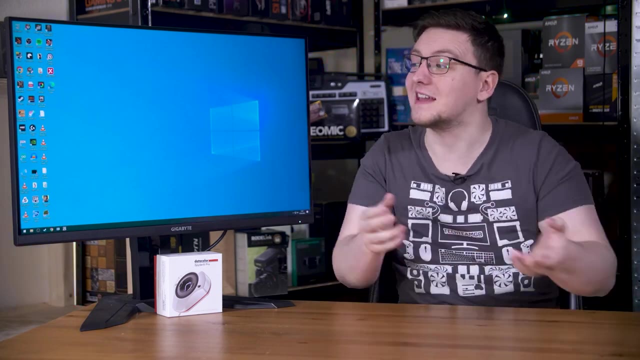 Basically a tool like the SpyderC records how off your display is with each of the colors and then saves a calibration file to your graphics card. That means when your graphics card goes to draw a new frame it distorts the true colors. to effectively cancel out the inaccuracies of your monitor's panel- Say your monitor- 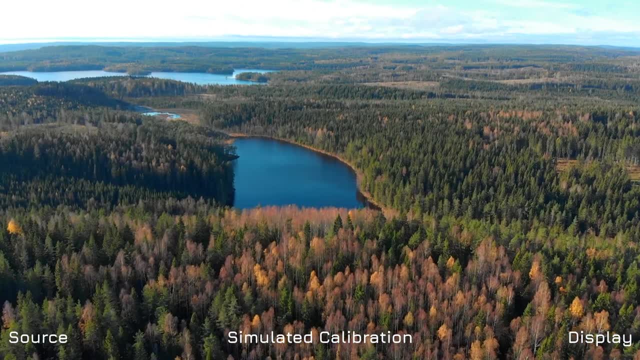 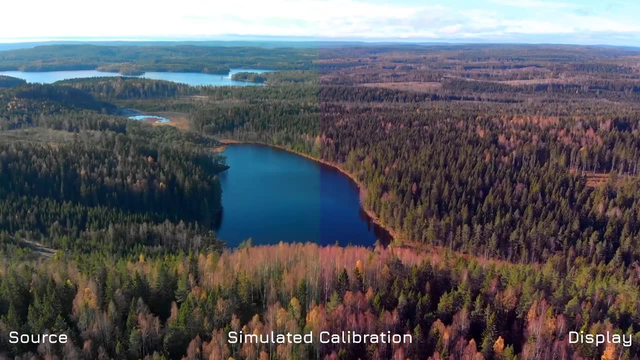 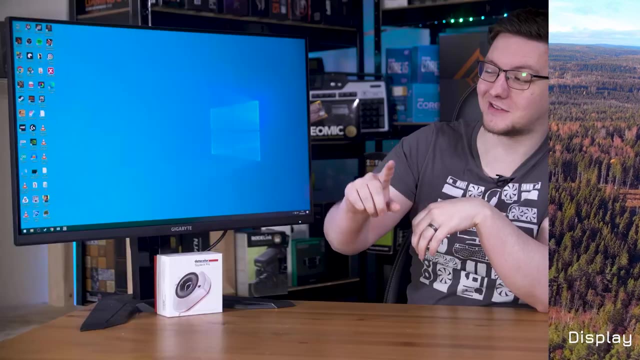 constantly shows slightly too much green. Well, your graphics card will tone down any green values to compensate. so what you see is accurate, but it's a bit of a trick to make your monitor display more accurate colors. That also means that that calibration only works with the system that you've.